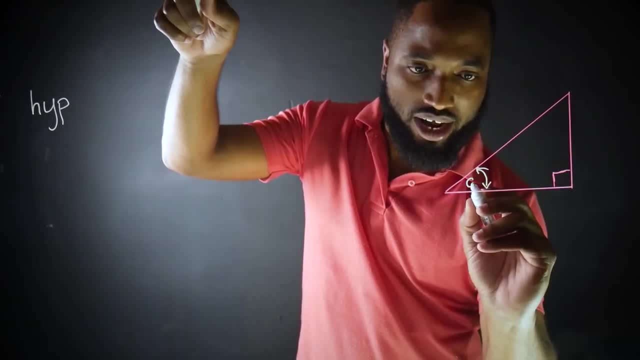 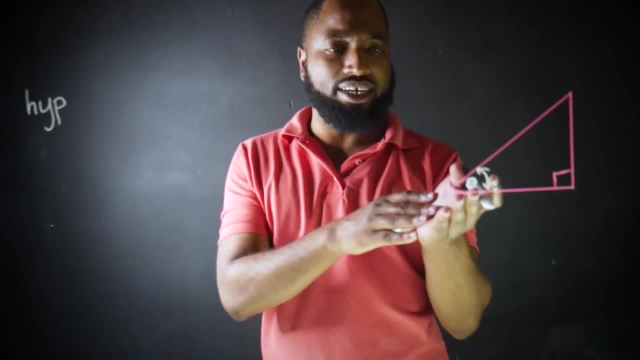 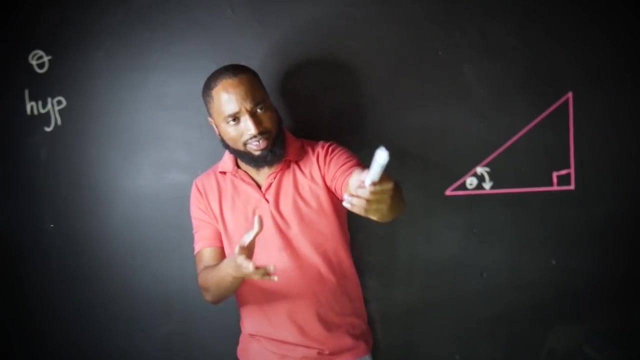 add in an angle, Let's call that angle theta. Theta is a symbol that looks like well, that We are just using to mean that angle. So since we named that angle theta, The angle theta, the opposite theta, we are gonna call the side opposite theta. 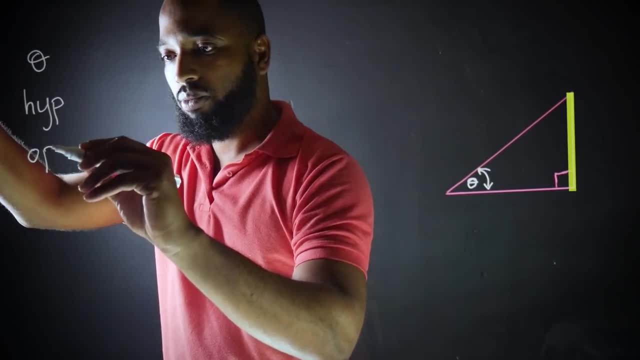 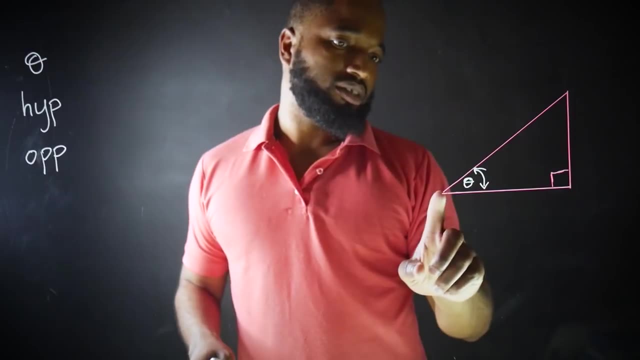 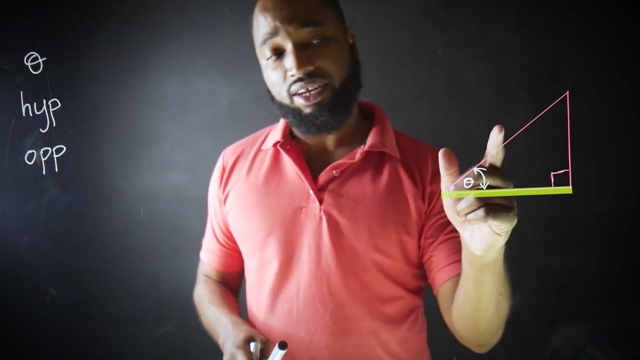 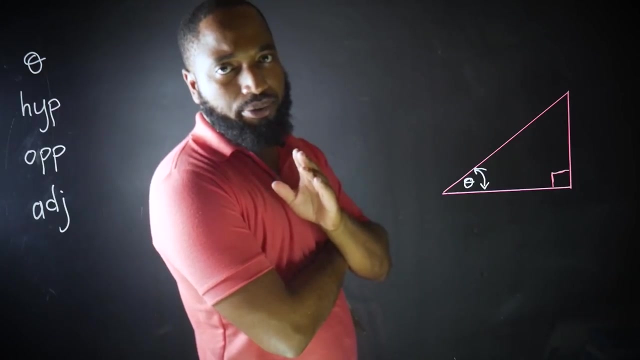 the opposite: OPP for opposite, HYPOTENUSE and opposite. That leaves you. You call the side the adjacent, because it's 求 right next to the angle. it's not the hypotenuse, but it's adjacent to the angle. so we call that the adjacent- ADJ for short. now, now let's explain. 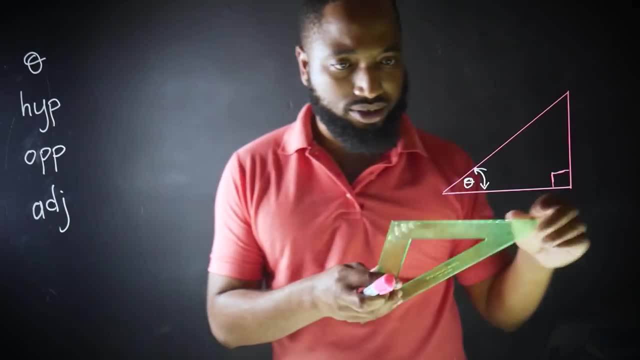 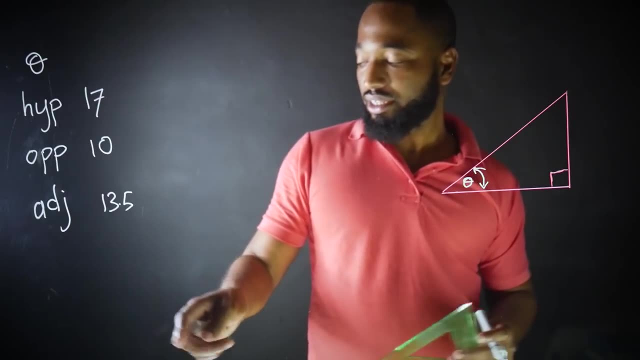 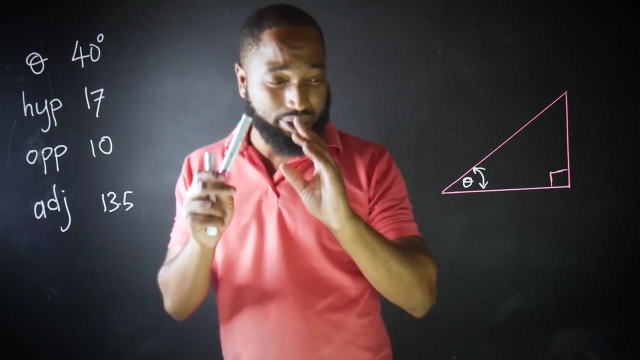 something you may not have noticed before. let me measure this adjacent opposite hypotenuse. these are the approximate lengths in centimeters of each side. the angle theta is approximately 40 degrees. now for the awesome part. if I take these numbers and apply to these ratios, I get these. 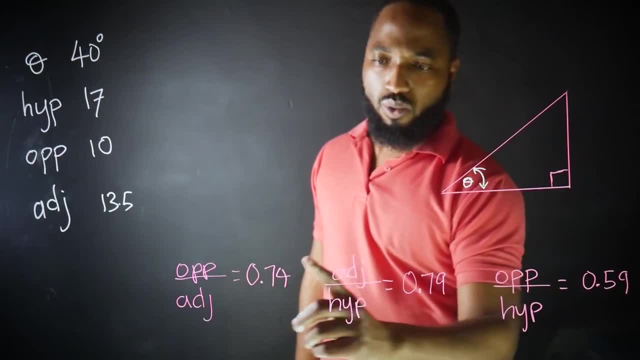 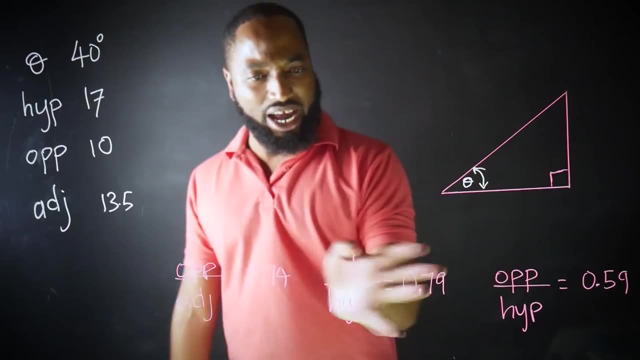 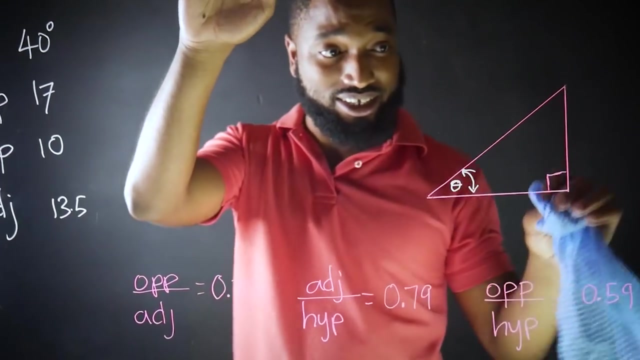 answers. well, they are approximated. the opposite over the hypotenuse was 10 over 17, approximately 0.59, and so on. the crazy thing about this that I noticed back in school that helped me understand this is that if I erase this part of the 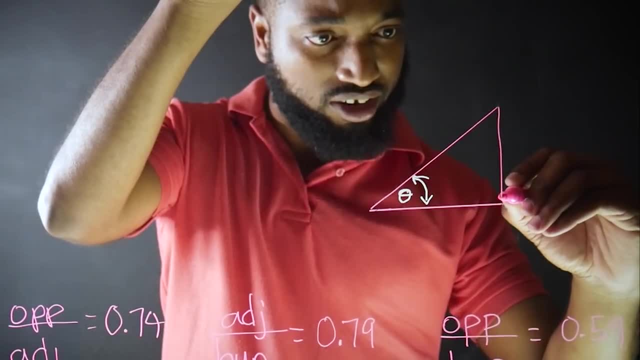 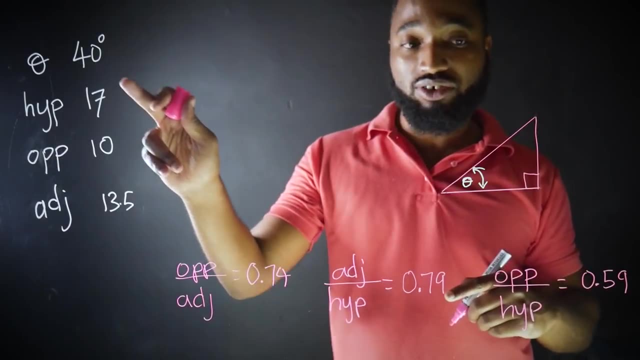 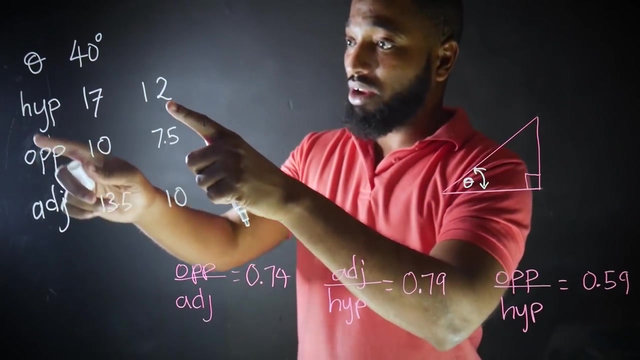 triangle here and made the triangle shorter so that it remains a right angle triangle with the same theta, with the same angle, here being 40 degrees. the sides of the triangle will change. the values will change to these new values, hypotenuse being 12, opposite being 7.5. 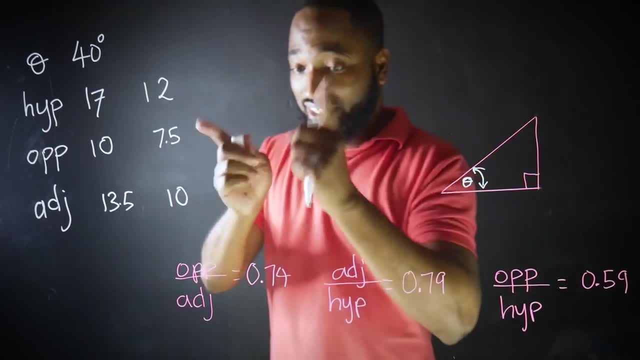 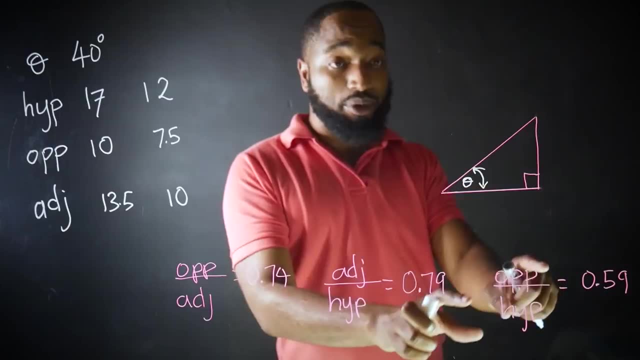 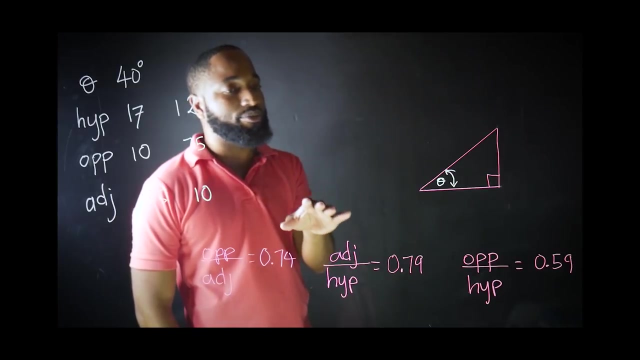 adjacent being 10. they got smaller, but the ratios of the sides remain the same. if I put these into these formula: approximately, approximately, earlier, approximately. this is all we want to check for later. to make sure, approximately, the diagram could be a little so. what you're saying is that it doesn't matter the size of the 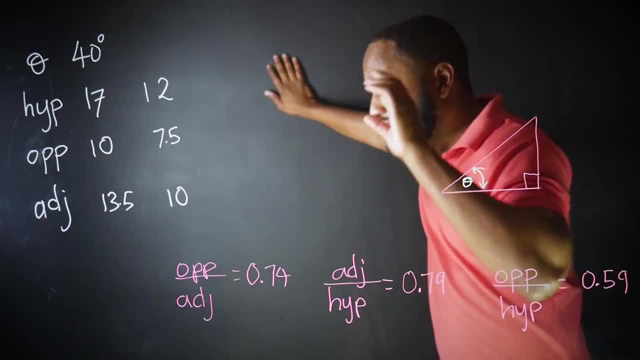 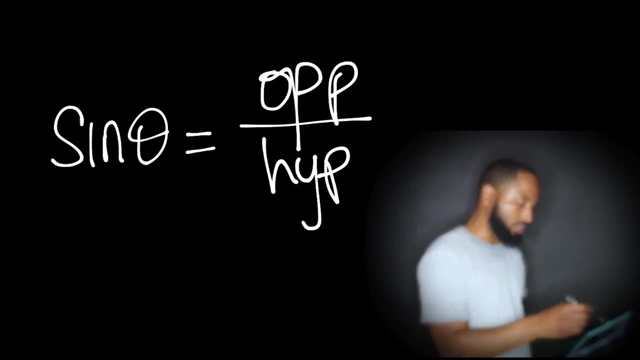 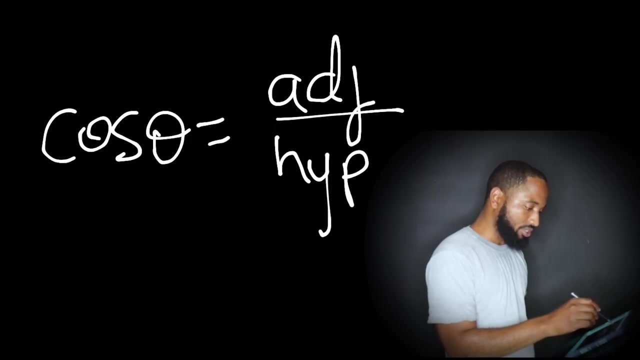 right angle triangle. once the angles remain the same, the ratios of the sides remain the same, yep, and of course you need to know what it represents and your ratios. our sine is the opposite over hypotenuse. cosine of theta here is adjacent over hypotenuse and our boy, 10 is. 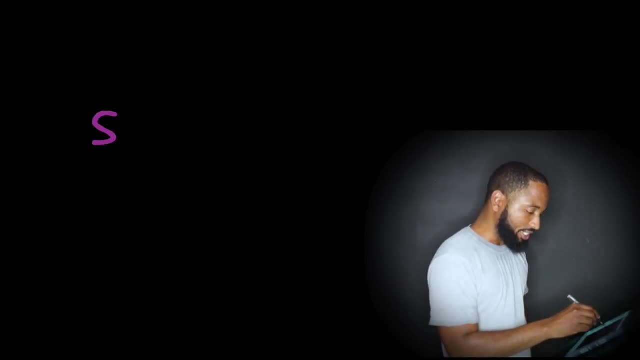 opposite over adjacent. And, of course, the common saying that we use to memorize, that is: SOHCAHTOA: Sine is opposite over hypotenuse, Cosine is adjacent over hypotenuse, Tangent is opposite over adjacent. So that's the acronym you can use to memorize that Question time. So let's 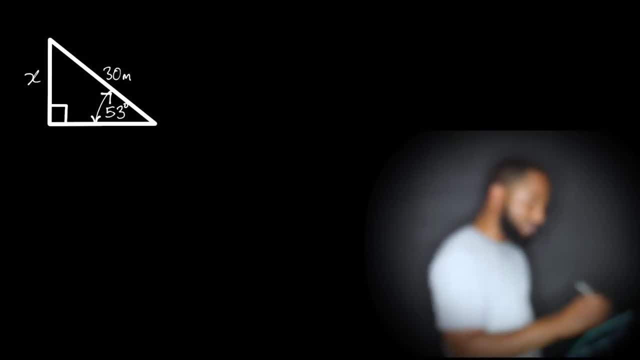 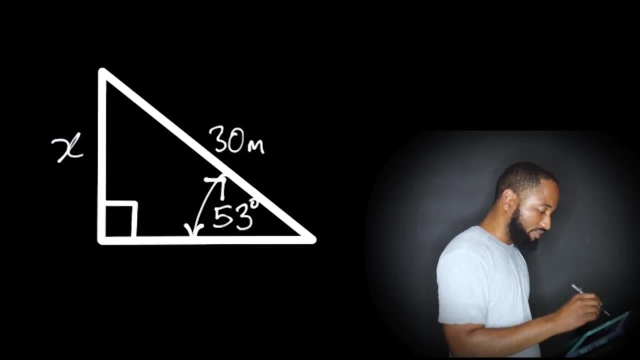 start off with an easy question. The first thing you need to always identify is what we're trying to find. We're trying to find this side here, X, And what sides will we be given? Well, we have the angle, And this is opposite the angle. So that's the opposite. 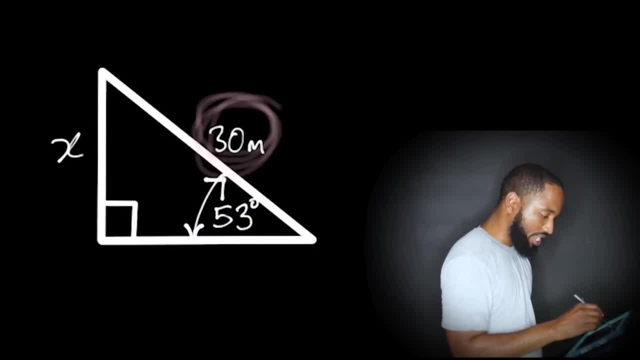 And this guy over here, This guy That's the longest side. So that's the hypotenuse. So we have the hypotenuse and the opposite. So that means we've got to use sine theta equal opposite to hypotenuse. And then you go to your substitution line, The fifty three. It 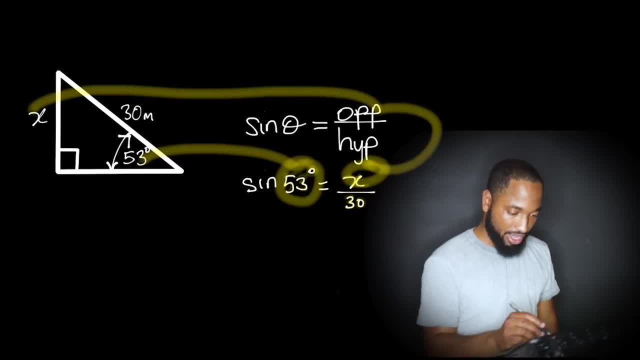 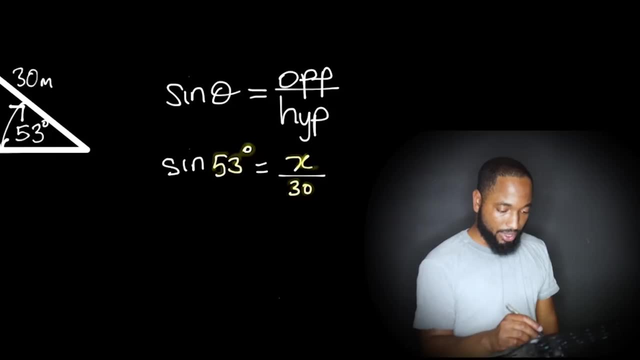 is the angle, X is the opposite, which is here, And we have titty, which is the hypotenuse, which is here, Longest side, Sine, opposite the right angle, And some simple algebra will get you down to. X is equal to titty times sine fifty three, because the X is on top. so 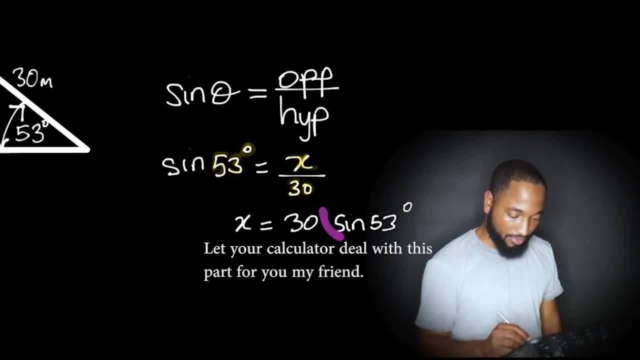 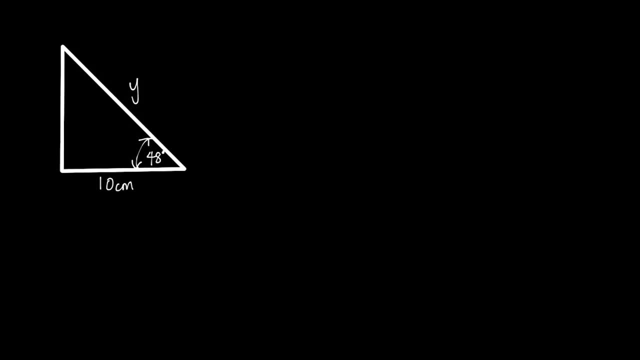 when you're talking about titty, it tends to multiply, So you can think of it as having a multiply sign right there. So in the end, X is equal to twenty four meters. That's easy, right? Let's look at another one. Alright, so this is simple as well. Let's find out. 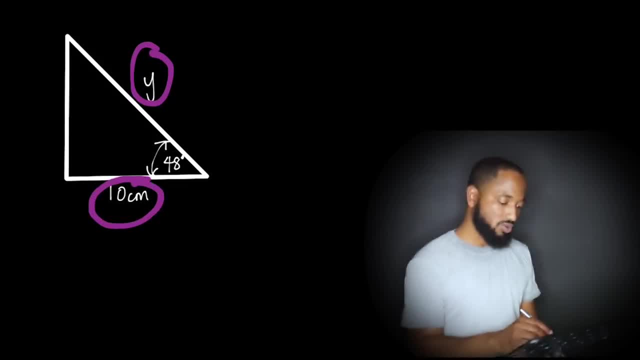 what size we give him. We have the hypotenuse, We have the. who are you? You are right next to the angle, You are at opposite. So you must be, You must be the adjacent. So we have the adjacent and the hypotenuse. Adjacent and hypotenuse, that's ka from the, so ka to. 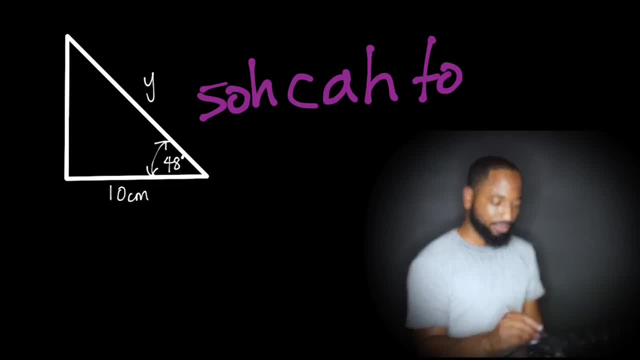 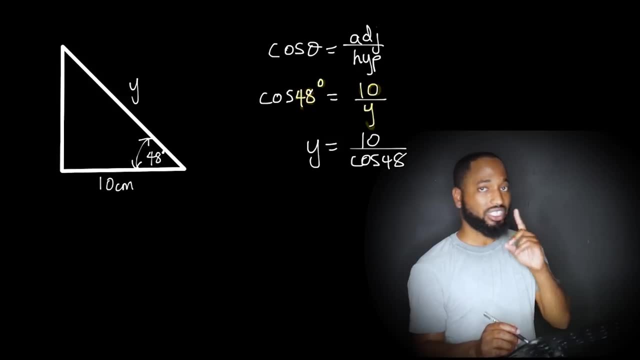 wa. So we're going to use cosine right. Start off with cos. theta is equal to adjacent to hypotenuse. Start off with the formula Substitute, Rearrange This time, since the Y is on the underneath it. It comes out like this: when we rearrange and do our little algebra, You can think of this: 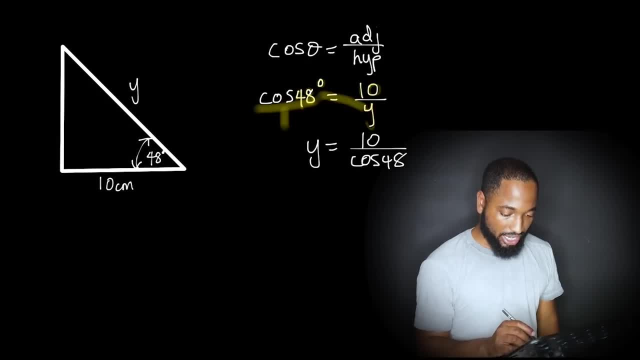 as if it was over one Cos forty eight over one, And there's a kind of multiplying scene and then a dividing scene going on here. So you'll end up with ten over cos forty eight. We call that in your calculator. you get around fifteen centimeters Normally, you approximate. 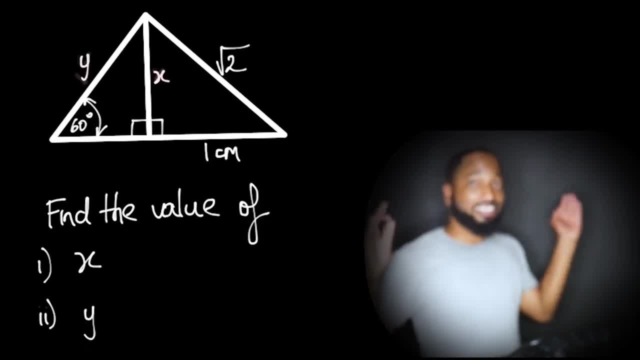 the three significant figures, one decimal places when you're doing trigonometry. This next question is a bit more challenging. We're going to combine some stuff we learned in the last video on Pythagoras Theorem. Make a check that out. So we need to find X, then we need to find Y. X is here, Y is there, So 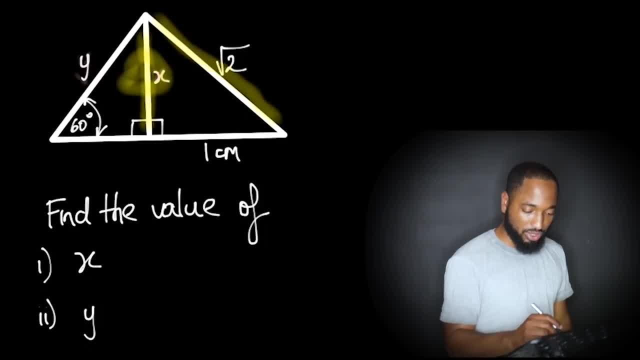 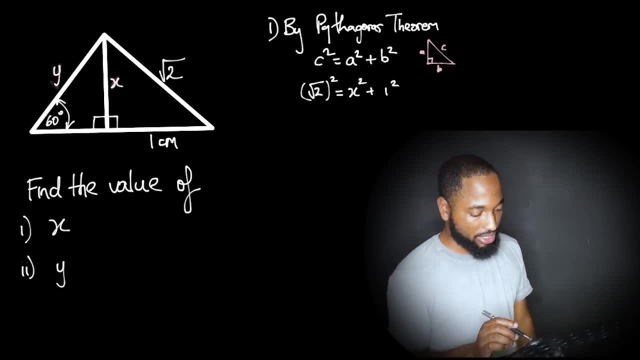 X looks like a Pythagoras Theorem question because there's a hypotenuse and the other two sides there, So we just hit them a little. Pythagoras there now, buddy. By Pythagoras Theorem, C squared is equal to A squared plus B squared. Substitute here This is C, here represents: 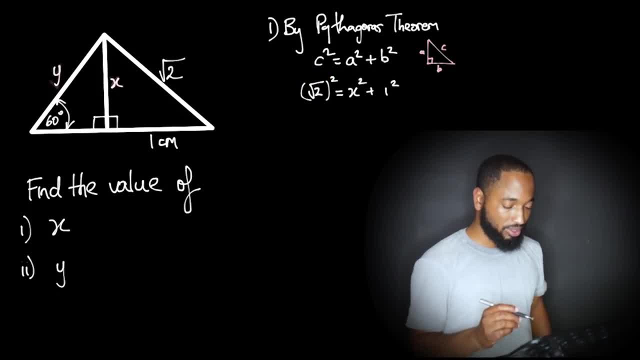 the hypotenuse squared of two. So what are we doing here? We're going to combine some things we learned in the last video on Pythagoras Theorem. We're going to check that out. So of 2, square root of 2, sometimes they put seeds and stuff in this. AdMob students you. 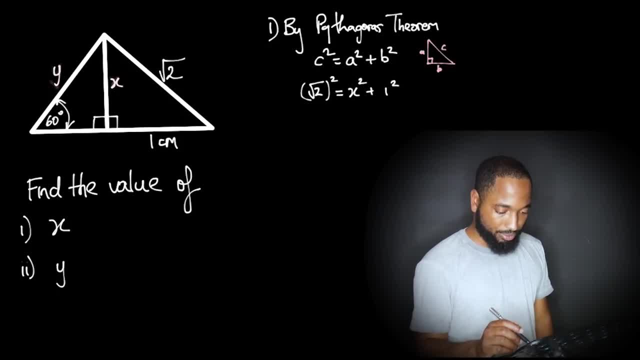 all should be able to walk through this. Then you go ahead and you get: x is equal to 1 as well, and this is a common triangle that all AdMob students should know about. We use this to prove what the sine and cos of 45 is. Okay, so we have x. now to find y. y is. 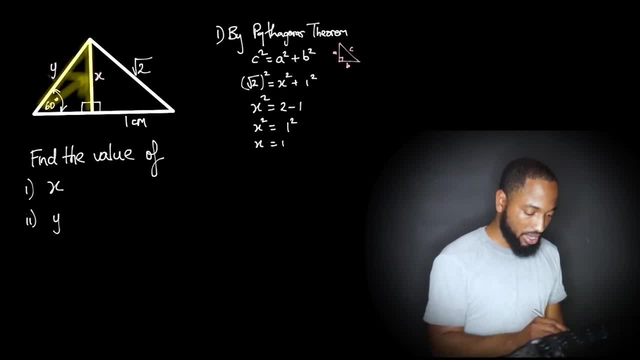 formed by noticing that we have the opposite of this and we have the hypotenuse on this side, Opposite hypotenuse. What ratio are we going to use? What ratio are we going to use Sine? Sine 60 is equal to the opposite of hypotenuse. 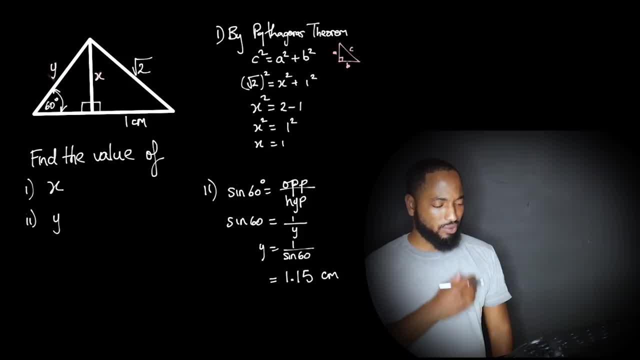 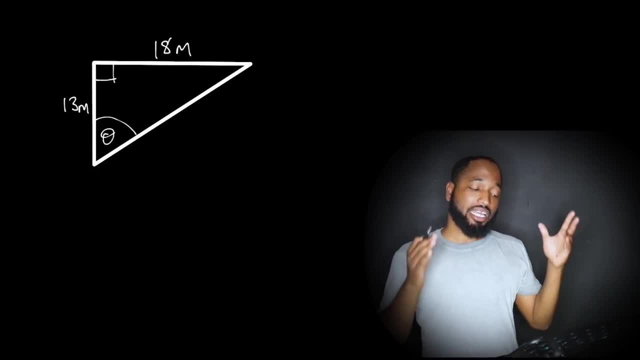 We'll get out and you get: y is equal to about 1.15, or you should get something like 2 over the square root of 3 or something. so What about a question like this? The angle this time is unknown. We again.